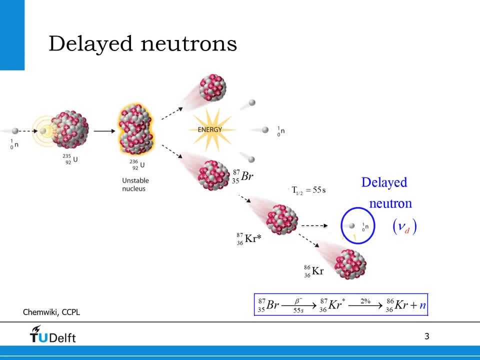 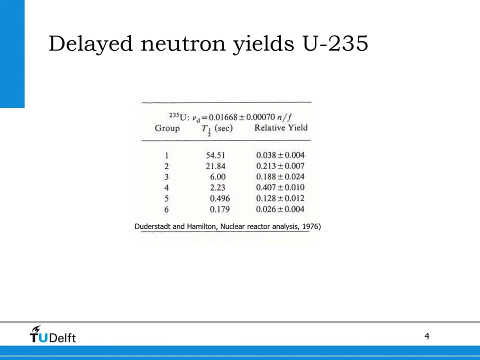 products that emit a neutron in the decay chain are called precursors. By definition, each precursor atom emits one delayed neutron in the decay chain. The number of delayed neutrons in the fission process of uranium-235 equals, on average, about 0.017,, which is a very small number compared to the number of prompt neutrons of about 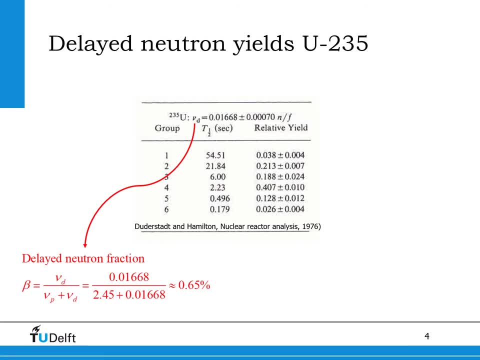 2.45.. The fraction of delayed neutrons of uranium-235 is only 0.65%, as shown in red on the slide. The table shown shows the split-up of the precursor in six families, but sometimes in other datasets, eight families are used. 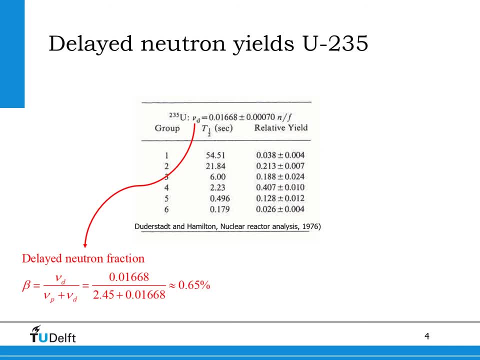 The half-life of the precursors of uranium-235 range from 0.18 to 55 seconds, and the latter is mainly due to the decay of the bromium to krypton that we've seen. On average, it takes about 13 seconds until the delayed neutron is emitted. 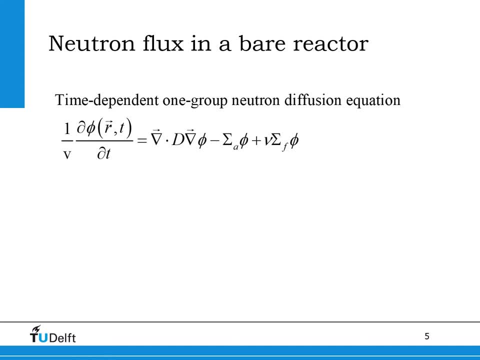 To derive the so-called point kinetics equations, we start with a one-group time-dependent neutron diffusion equation. for a neutron flux, phi, The V on the left-hand side of this equation is a neutron velocity, while the first term on the right-hand side of this equation is a neutron leakage rate in the fusion theory. 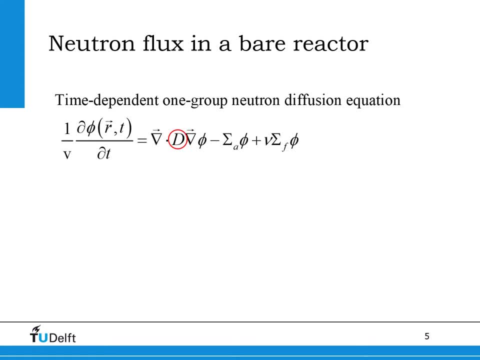 with capital D, the neutron diffusion rate. The first term on the right-hand side of this equation is a neutron leakage rate in the fusion theory, with capital D, the neutron diffusion rate. The second term is a neutron absorption rate with sigma A, the macroscopic absorption. 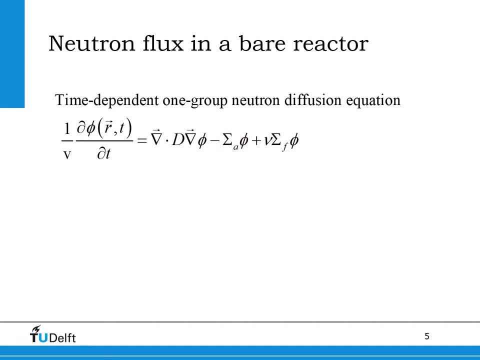 cross-section, and the third term is a neutron production rate due to fission, with sigma F, the macroscopic fission cross-section, and nu, the total number of neutrons per fission event. Note that nu is the sum of the prompt and delayed neutrons per fission. 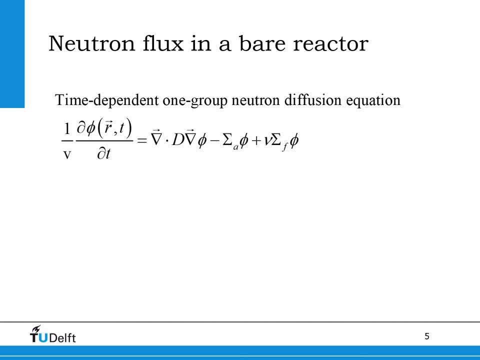 The resultant of these three terms determine if the neutron flux phi is a neutron leakage flux increases or decreases in time or remains stationary. To solve this equation we need boundary conditions For a bare geometry. this is given in the fusion theory by putting the flux to zero. 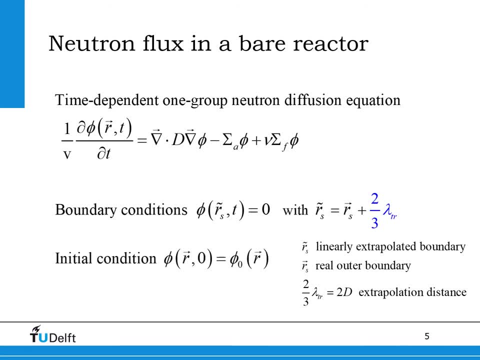 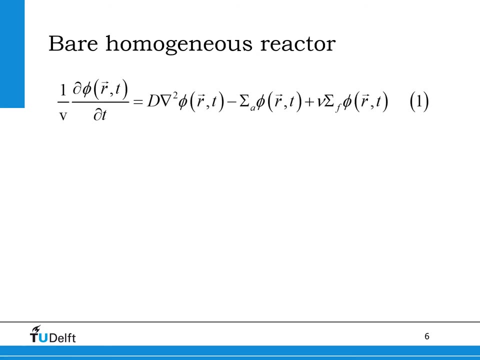 at a linearly extrapolated boundary. We also need initial conditions. This implies that the neutron flux should be given at some time. t here indicated with time, t is zero. Here the time-dependent diffusion equation is shown again, but now with the diffusion. 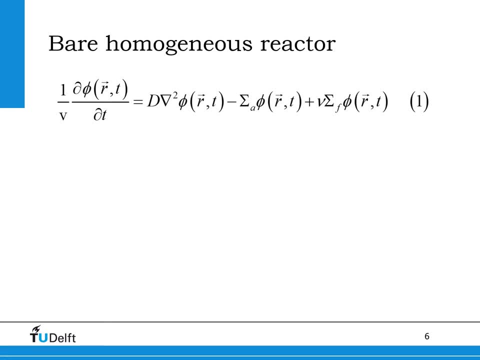 coefficient in the first term on the right-hand side, before the divergence term. This is valid if the composition of the reactor core is homogeneous. In the derivation of the point kinetics equations, we also assume that the flux in the reactor core is in the fundamental mode. 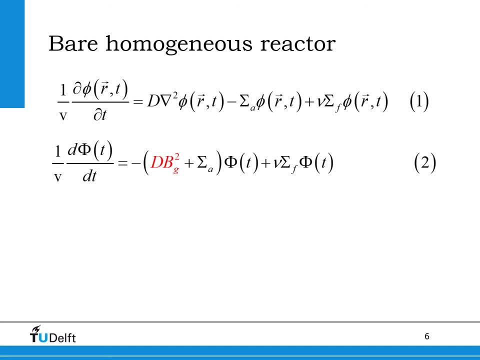 This implies that the leakage term can be rewritten in terms of the geometrical buckling as shown in red in equation two. In this equation we have also integrated the neutron flux over the whole volume of the reactor core. This total neutron flux is indicated with capital phi and is only dependent on time. 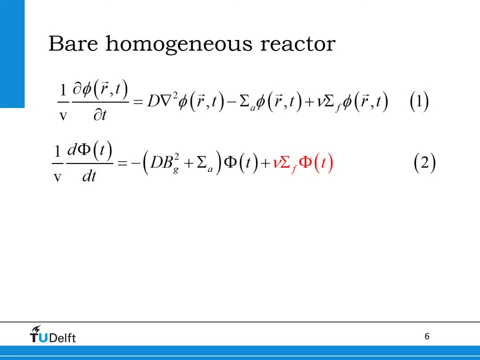 Now we must realize that the production of neutrons in a fission process consists of the prompt neutrons released promptly at the fission event and the decay of precursor atoms. The prompt neutron production rate equals νp times the macroscopic fission cross-section. 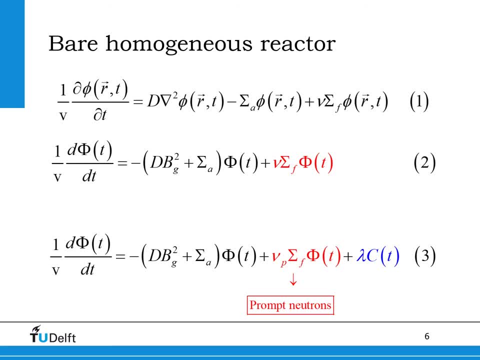 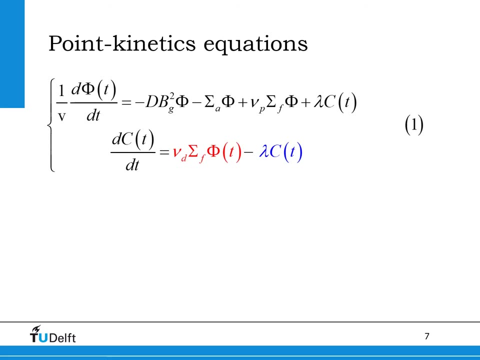 times the total neutron flux and is shown in red in equation 3.. As said before, each precursor atom releases one delayed neutron upon decay. This term is shown in blue in equation 3.. Of course we need an additional equation to evaluate the number of precursor atoms. 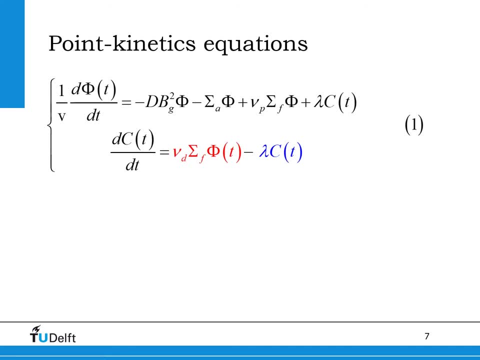 in the reactor core as a function of time. This is shown in the second equation on this slide, where the red term describes the production of precursor atoms, which is proportional to the fission rate in the core, and the blue term describes the removal of precursor atoms due to decay. 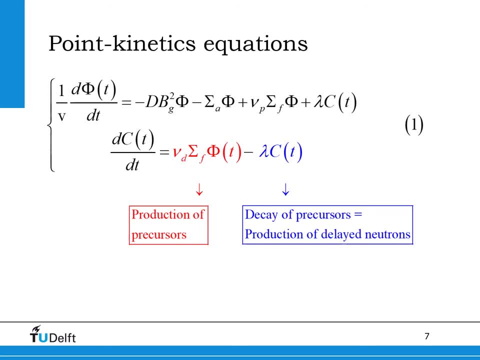 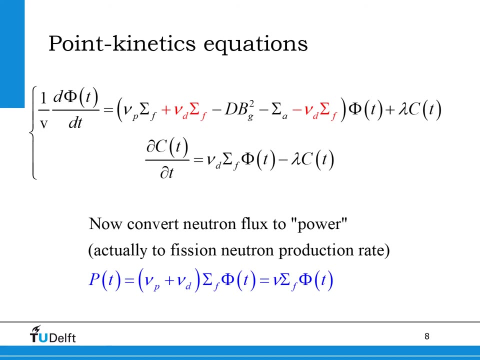 Of course, when a precursor atom decays, a delayed neutron is produced, because by definition each precursor atom produces exactly one delayed neutron. We now recast the fission term in the first equation a bit by adding and subtracting νd times the macroscopic fission cross-section on the right-hand side. 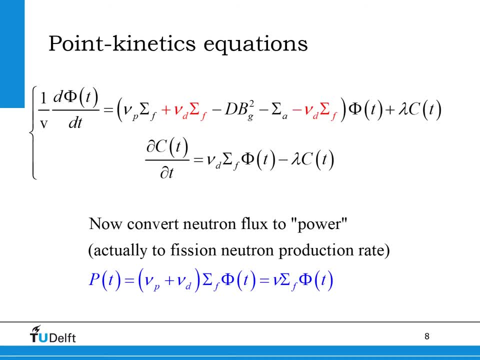 On the next slide we will convert each term containing the total neutron flux to the total fission neutron production rate, which is shown in blue at the bottom of this slide. The total neutron production rate is proportional to the fission rate in the core and therefore 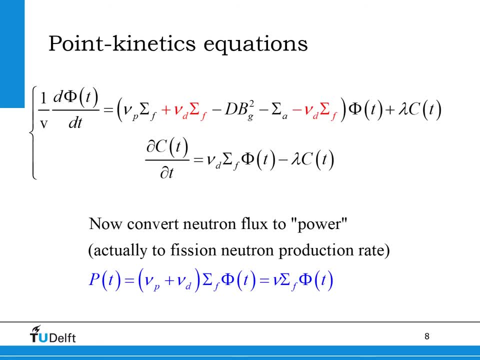 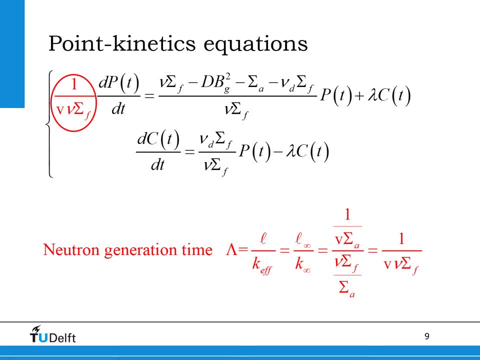 also to the total power produced in the core. This set of equations are the same as on the previous slide, but now with the total neutron flux converted to the fission neutron production rate in the core. The term in red on the left-hand side of the equation is called the neutron generation. 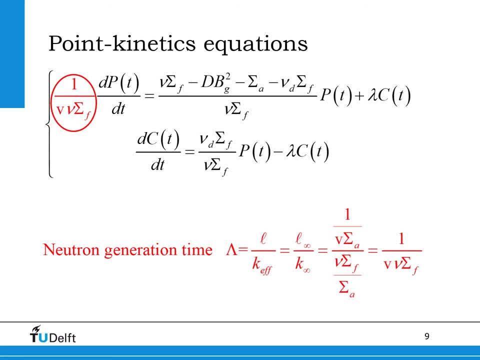 time and is a prompt neutron lifetime. The current time of the neutron generation is the current time of the fission neutron production rate, which is the average time L divided by the effective multiplication factor k-effective and has a meaning of the average time needed for a neutron to create. 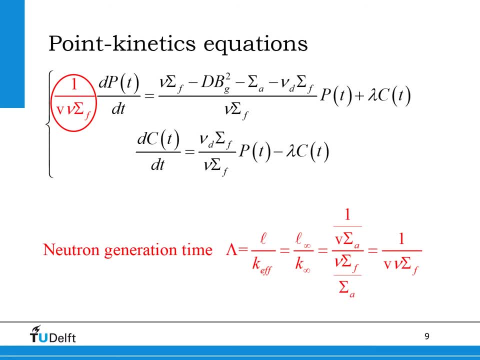 one new fission neutron. The red-colored term on the right-hand side can be rewritten using the reactivity of the reactor core. To derive an expression for the reactivity, we first divide the red terms by the mass of neutron, which we define as the mass of neutron. 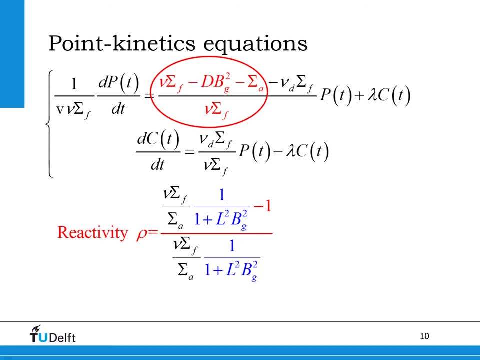 The material part is shown at the bottom of the slide- by the single反ong equation which we have written out, and by the spectroscopic absorption cross-section, and then by 1 plus L squared, b squared. These are the blue parts in the equation at the bottom of the slide. 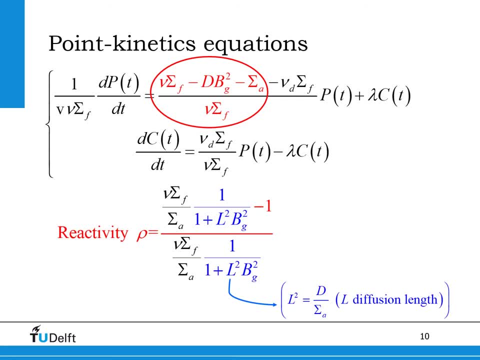 In other lectures on the criticality condition of bair homogeneous reactor cores, we have demonstrated that the blue part represents the non-leakage probability of the reactor core, a multiplication factor of an infinitely large reactor core, also called k-infinite. And finally, we can rewrite the product of the infinite multiplication factor and the 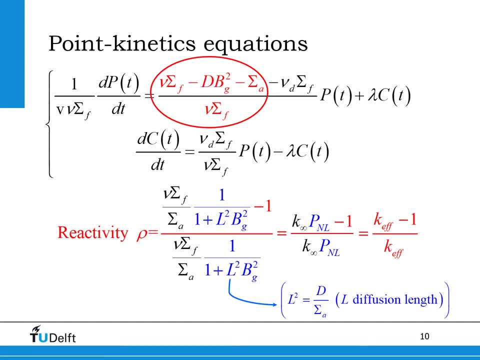 non-liguid probability as the effective multiplication factor of the reactor core. Using these formulations we see that the reactivity of the reactor core equals the ratio of the effective multiplication factor minus one divided by the effective multiplication factor. In the equations we see also the ratio of the production of precursor atoms nu d times. 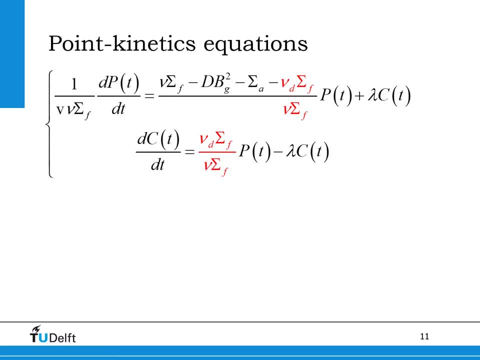 the microscopic fission cross-section and the total fission neutron production shown in red on this slide. This ratio is called the delayed neutron fraction And is usually given the symbol β. Note that the precursor atoms only emit a delayed neutron several seconds after the. 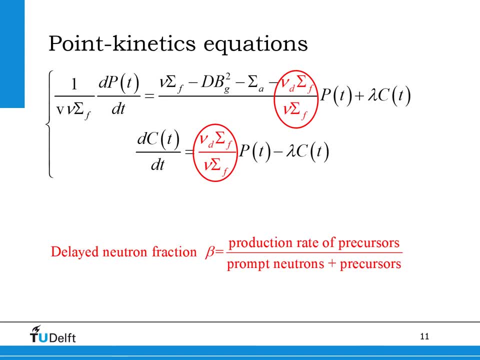 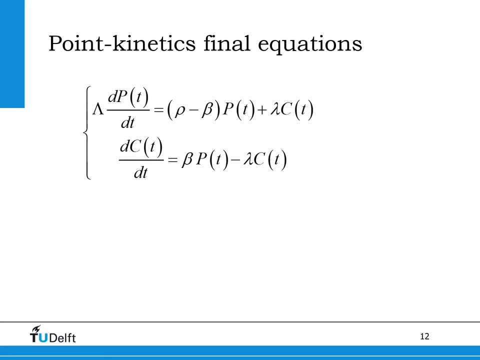 fission event itself. The equations on this slide give the point kinetics equations for one family of precursors. It's a coupled set of equations, one for the fission neutron production rate, P, and one for the precursor atoms C, In case we want to include more families of precursors in our point kinetics equation. 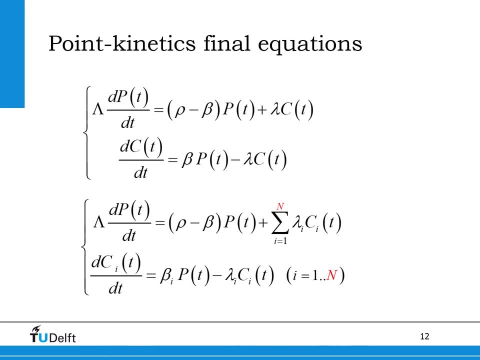 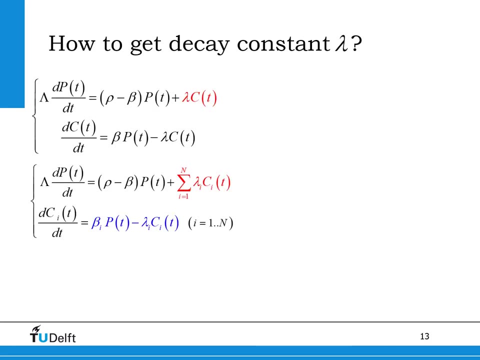 we have to include each family separately and also write a balance equation for each family. This is shown in the set of equations at the bottom of this slide. The number of families can be 6 or 8.. From these set of point kinetics equations we can derive the effective decay coefficient. 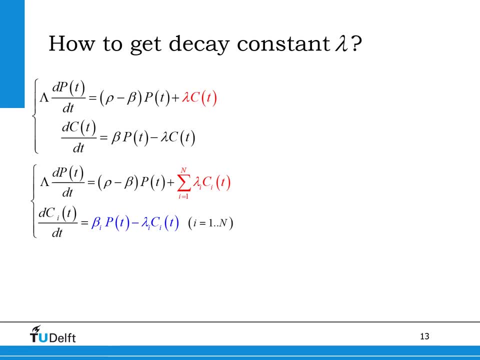 When we lump all precursor families into one. First, note that the red term in each equation for the fission neutron production rate P need to be equal to each other. From this we can extract the equality shown in red. Secondly, in a stationary reactor the total number of precursor atoms does not change. 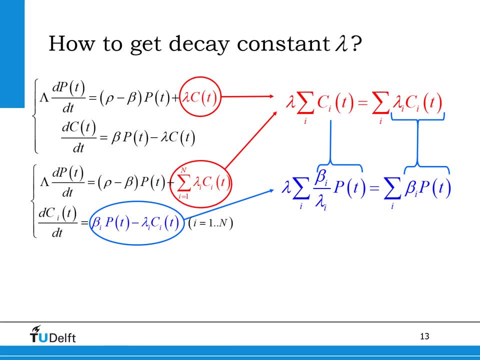 in time. Using this we can derive the equation in blue And from this we can derive the final number of precursor atoms, The final expression for the decay constant lambda, in case we have only one family of precursors. If we insert the values for beta and lambda for each precursor family of uranium-235, as 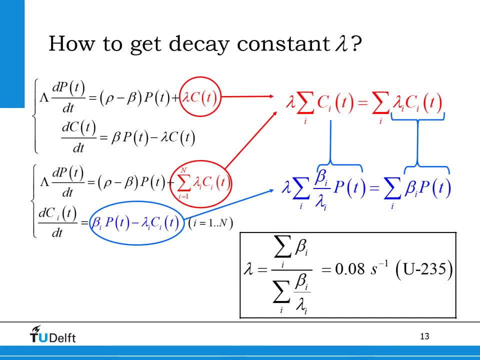 shown on slide 4 of this presentation, we can get for lambda a value of 0.08 per second, And this means that on average, a delayed neutron is emitted 13 seconds after a fission event. This is 1 divided by lambda. 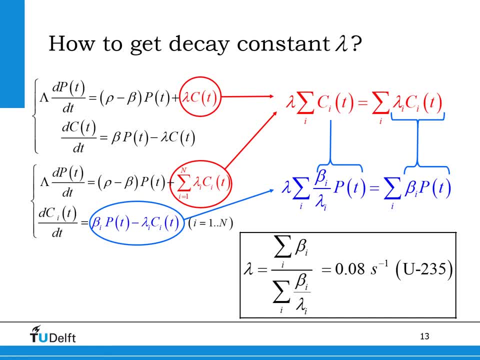 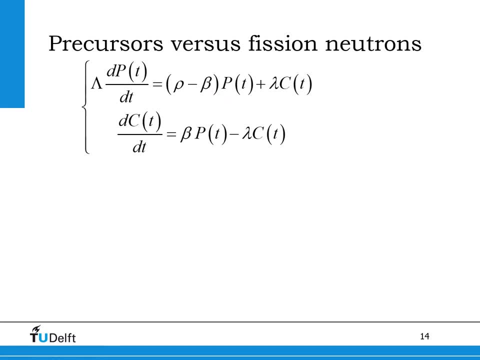 And this means that, on average, a delayed neutron is emitted 13 seconds after a fission event. It is interesting to calculate the number of precursor atoms in the fuel and to compare these with the number of neutrons in the reactor core. Assuming a stationary situation, we can derive from the second equation an expression for: 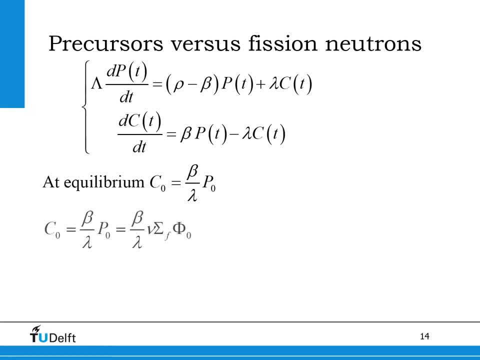 the precursor atoms. as shown on the slide Inserting the expression for P0,, which is a stationary fission neutron production rate in the reactor core, We get that the number of precursors in the fuel is beta divided by the decay constant of the lumped precursor family, divided by the neutron generation time times the number. 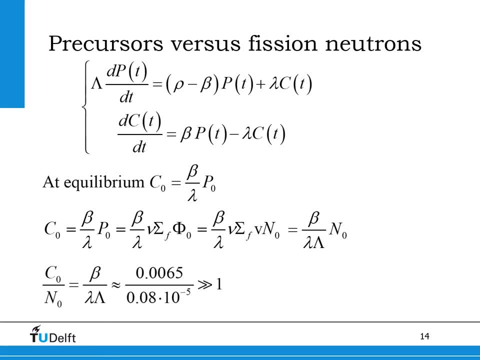 of neutrons in the reactor core. Because the neutron generation time can be of the order 10-5,, the resulting number is typically much smaller than unity, which means that the fuel contains many more precursor atoms than the number of free neutrons. 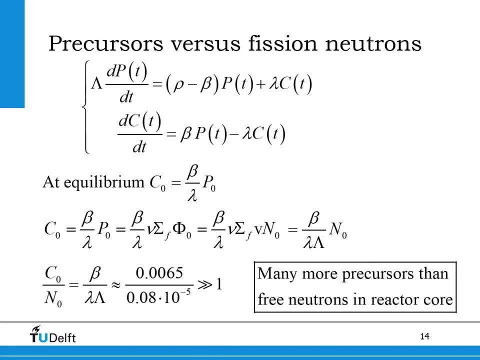 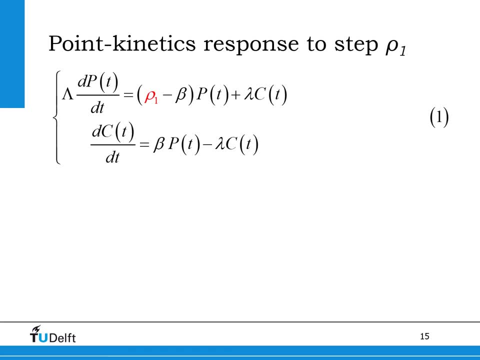 The result is that the fuel contains many more precursor atoms than the number of free neutrons in the reactor core. Now we will solve the point. kinetics equations for a step function in the reactivity of the core. Assume the reactivity increases with the value of ρ1 at time t0. 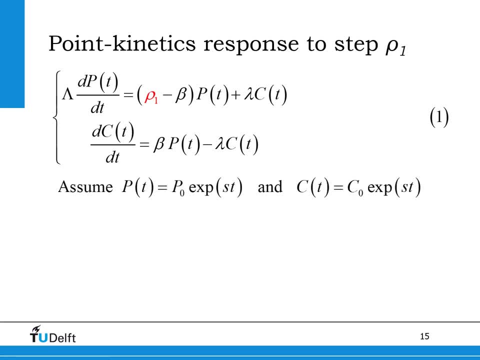 We will try to find a solution by inserting an exponential function for P and C, as shown on the slide. The solution is the set of coupled equations with S as a parameter, as shown in equation 2.. Insert the equation for C into the first equation for P. We get an expression for P, as shown. 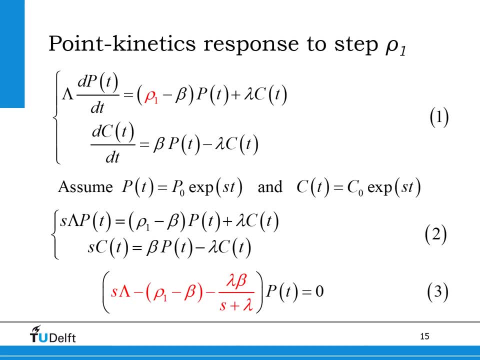 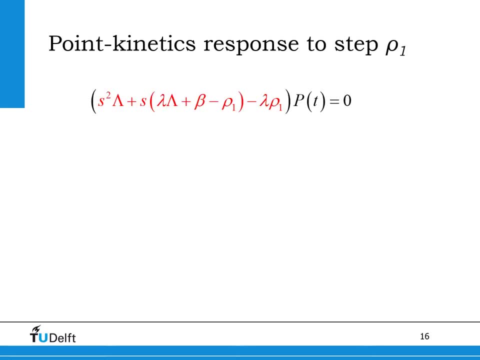 in equation 3.. Note that this equation has only a non-trivial solution if the polynomial in S equals 0.. Here we have given the same polynomial again. The two roots of this second-order equation are the same. The second-order equation has two roots. 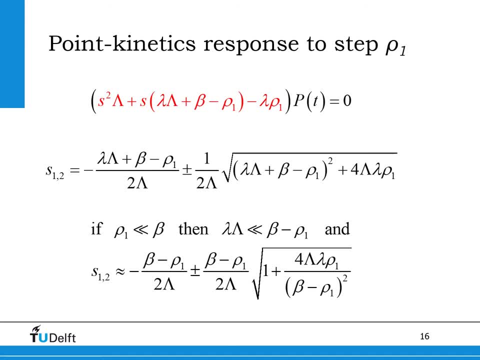 The second-order equation has two roots. The third-order equation has two roots, in addition to S and P. Now it is really simple. We can simplify the solution a bit by restricting ourselves to small reactivity steps. this means that rpm1 is much smaller than β. 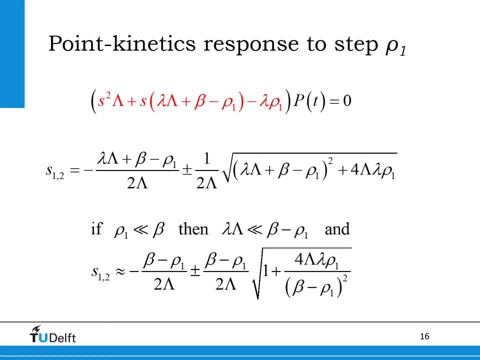 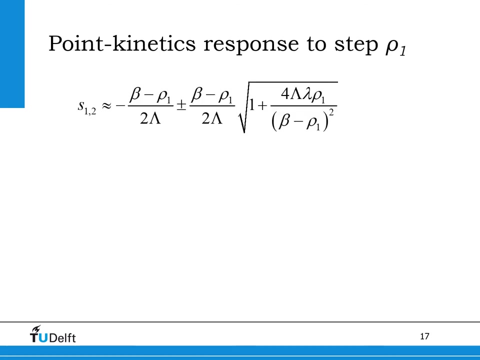 And assuming that the generation time is very small compared to β-rm1.. We then obtain the result for the two roots S도1 and S trendoR24, as shown at the bottom of the slide. Here we've shown the expression for the roots S1 and S2 again. 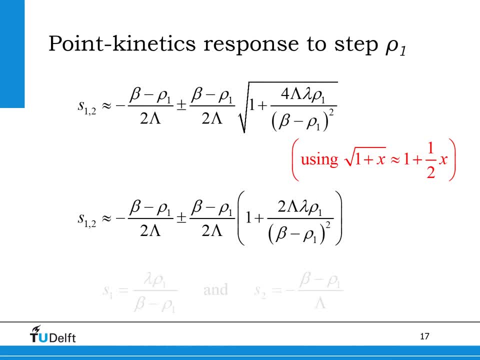 Approximating the root with the first term of the Taylor expansion, we can get the final values of S1 and S2 as shown on the slide. For small values of the reactivity, S1 is almost proportional to the reactivity and it has always the same sign as the reactivity. 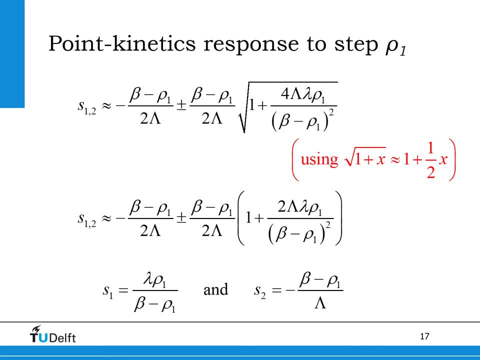 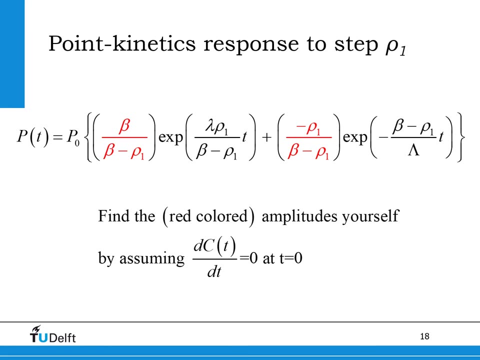 While the value of S2 is always negative and because the generation time is generally very small, it always has a large negative value. The formula on this slide gives the final expression for the fission neutron reduction rate as a function of time. after assertion of a constant reactivity, rho1, at time t0.. 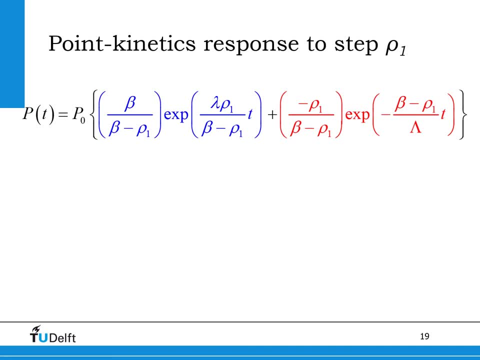 Thank you. In this plot the two contributions are shown. The first term in blue is a root corresponding to S1.. After a positive step in the reactivity, the fission neutron reduction rate jumps to a higher value and then increases exponentially afterwards. 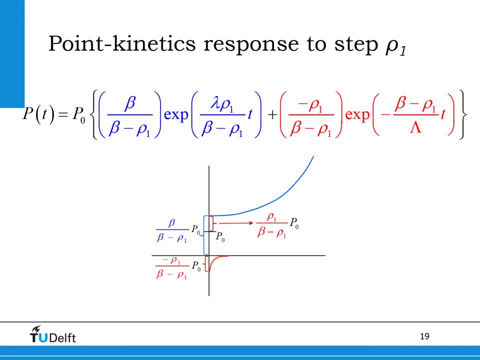 This is shown by the blue curve in the plot. The second term, corresponding to S2, is a small correction to the blue term. It corresponds to the response of the reactor due to the prompt neutrons. Note that if the generation time capital lambda would go to zero, meaning that the prompt 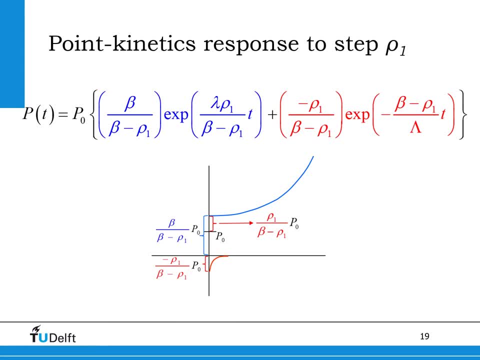 neutrons would respond infinitely fast. the second term would not be visible in the plot anymore and the response would be as shown in the blue curve alone. We will explain more about the point. kinetics response with zero generation time if we discuss the prompt jump approximation. 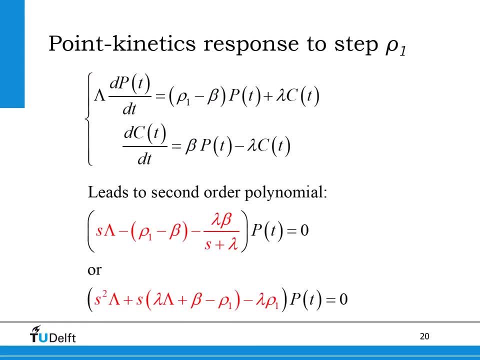 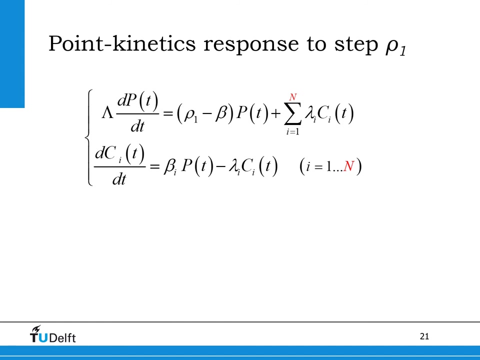 We have seen before that a point kinetics equation with only one group of precursor atoms leads to a second-order equation in S and thus to a solution of the fission neutron reduction rate containing two exponential functions. If we would start with the point kinetics equations with n number of precursor families, 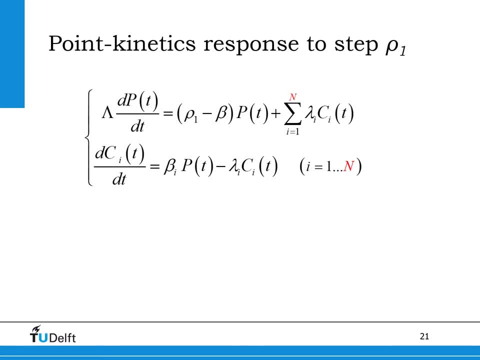 we would end up with the polynomial in S of order. We have seen before that a point kinetics equation with only one group of precursor families leads to a second-order equation in S of order. This is shown in the red formula at the bottom of the slide. 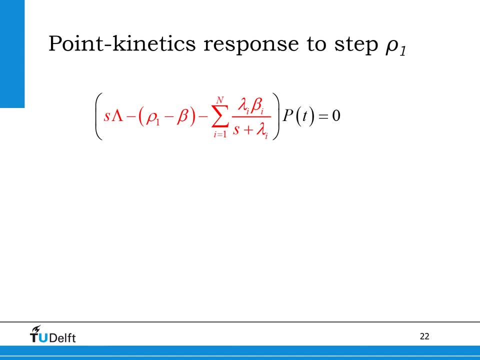 Here we have given the same polynomial again. Using the expression for the delayed neutron fraction, beta, as shown in black on the slide, we arrive at what is called in nuclear reactor physics the in-hour equation. This equation is shown in blue at the bottom of the slide. 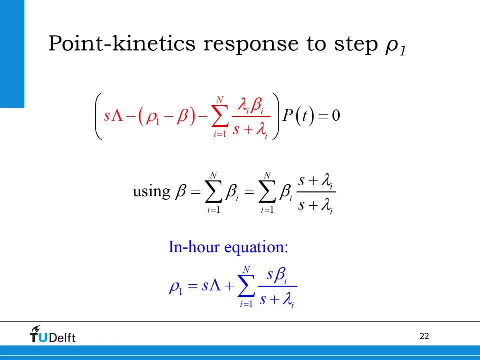 We have seen before that a point kinetics equation with only one group of precursor families leads to a second-order equation in S of order. Here we have given the same polynomial again, Using the expression for the delayed neutron fraction, beta, as shown in black on the slide. 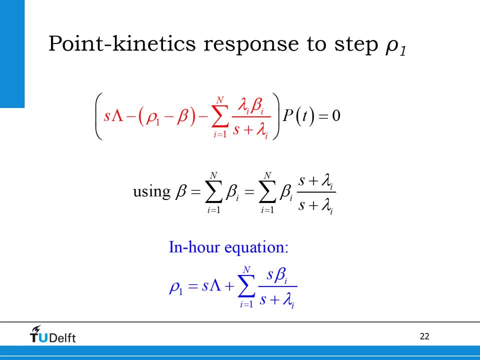 we arrive at what is called in nuclear reactor physics the in-hour equation. We have seen before that a point kinetics equation with only one group of precursor families leads to a second-order equation. in S of order, However, shown in black on the slide, we have introduced a labeling scheme where two 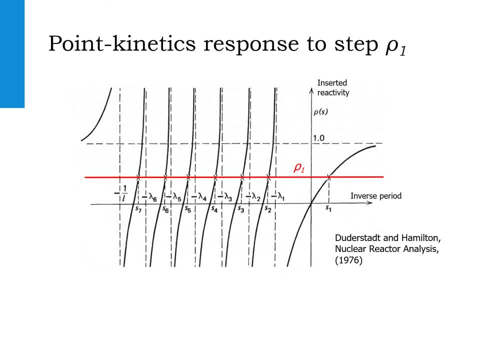 groups of precursors suits each other: E and R rates for Batman, E for Lin, E for E and R rates for E. As we completed, not first over the нимиnikations, we conclude that this equation means that are the cross points of the horizontal red line, which is the reactivity introduced with the curves. 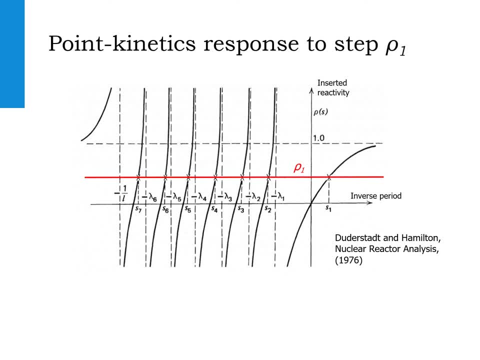 of the right-hand side of the in-hour equation. Note that for six families of recursive atoms, the solution of the in-hour equation counts seven roots in total. First, note that the reactivity can never exceed the value of unity. This means that the branch of the in-hour equation at the 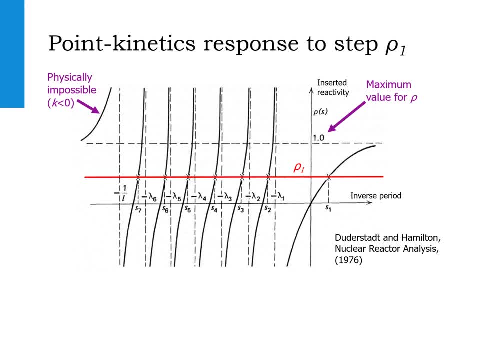 top left corner of the curve can never be reached. This region would actually correspond to a negative value of the multiplication factor, which is physically impossible. Only S1 has the same sign as the reactivity insertion itself. This is the blue curve on the right. All other S values are always negative and a corresponding exponential. 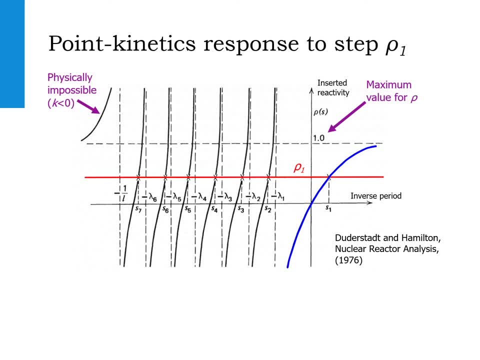 function in the solution for the power will always die out faster than the exponential function. The larger the reactivity insertion, the larger the value of S1 will be and the faster the power will increase. Theoretically, there is no limit on S1 at the positive side Note, however. 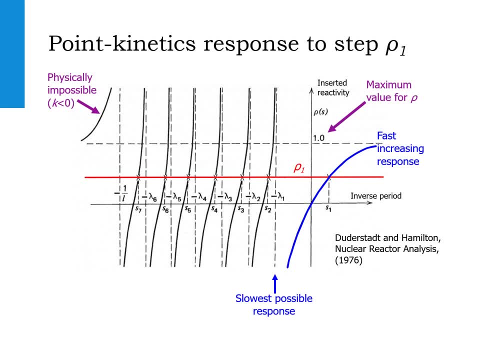 that the value of S1 for negative values is restricted. S1 can never cross the value of minus lambda 1, which is the decay constant of the longest-lived precursor atoms. This is logical: After a strong negative reactivity insertion, the precursors will continue to emit delayed. 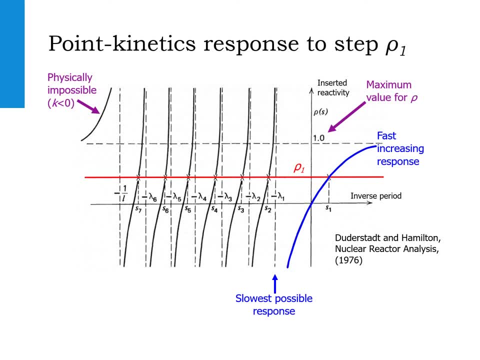 neutrons, and after all short-lived precursors have decayed. only the longest-lived precursors will dominate the time dependence of the reactor power. The long-term response of the reactor is then proportional to exponent S1 t. We can express this also in the reactor period, capital T. 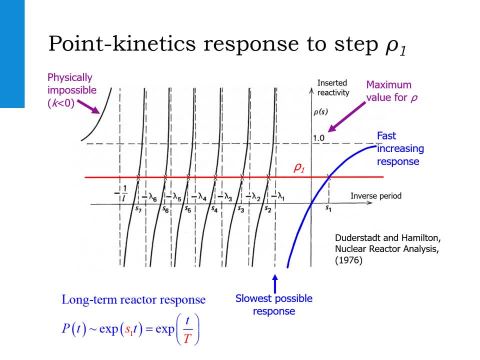 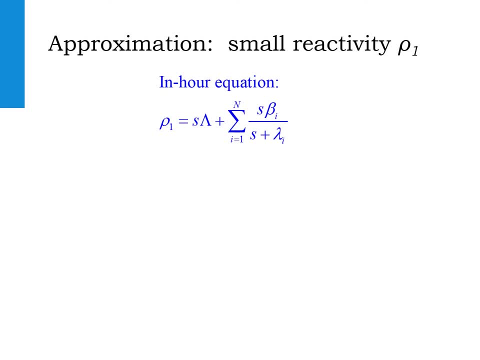 as shown in the formula at the bottom of this slide. We will now examine the limit of small reactivity insertions. Assuming that the reactivity inserted is much smaller than beta, the resulting magnitude of the S value will be much smaller than the lambda 1 value. 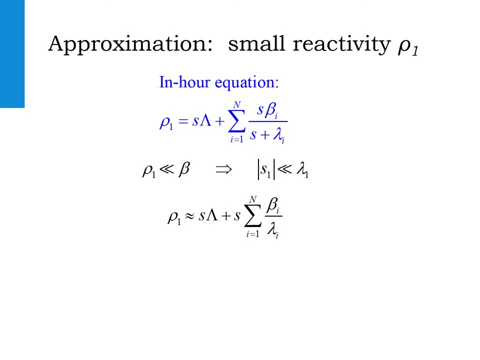 It's then easily seen that the reactor period capital T equals the effective neutron generation time, which is the neutron generation time, including the effect of delayed neutrons, divided by the reactivity insertion rho1.. This is approximately equal to the effective neutron lifetime divided by k-1.. 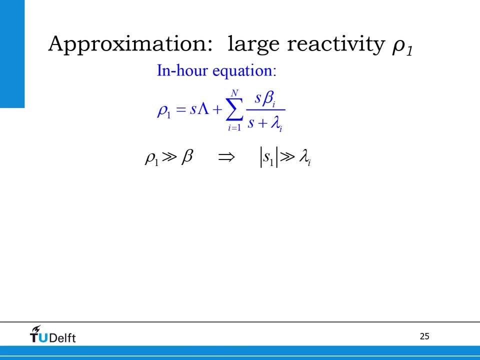 For very large values of the reactivity insertion, corresponding to values of the reactivity much larger than beta. the S-value is very large and positive because the reactor is now supercritical on prompt neutrons alone. it's in what we call the prompt supercritical state. 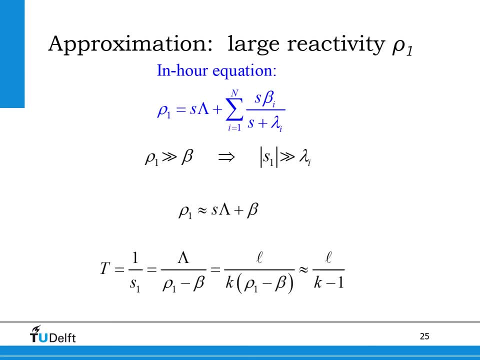 In this case, the reactor period equals the prompt neutron lifetime, L divided by k-1, and will in practice reach very small values, because L can be of the order of 1 to 10 microseconds. For sure, after such a large reactivity insertion. 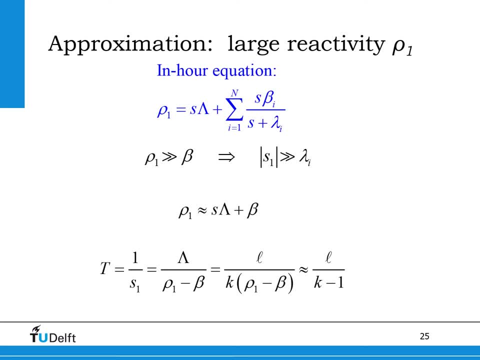 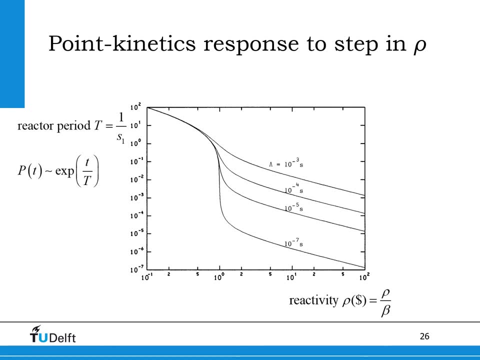 the reactor power will increase very rapidly. Here we've shown the reactor period- which is the inverse of S-1, versus the inserted reactivity. Note that we have given here the reactivity divided by the value of the delayed neutron fractions, which is usually called the reactivity expressed in units of dollar. 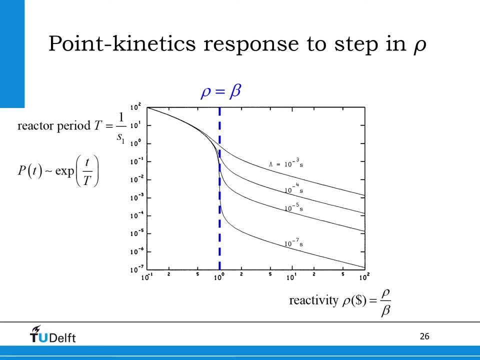 A reactivity of unity now corresponds to the value at which the reactor is critical on prompt neutrons alone. For small values of reactivity left of the blue dotted line, the reactor period becomes very large, which implies that the reactor will react mildly to the reactivity inserted. 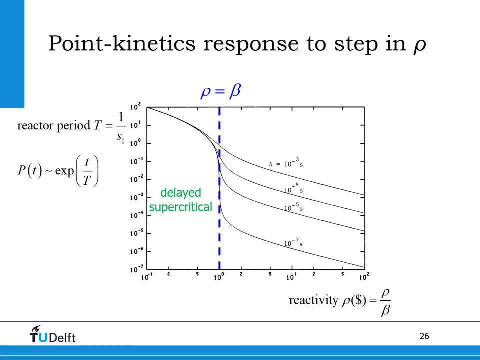 In this region. the reactor is easy to control and automatic feedback effects, like the nuclear Doppler effect, will easily and automatically compensate for the inserted reactivity. In this range the reactor is called delayed supercritical, and this is, of course, the only safe region to operate a nuclear reactor. 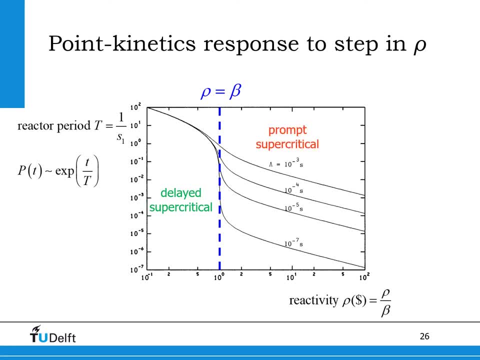 For values of reactivity larger than one dollar, the reactor becomes supercritical on prompt neutrons alone and the reactor power will increase very rapidly. The reactor period now depends strongly on the neutron generation time and for small values of the reactor, period becomes extremely small. 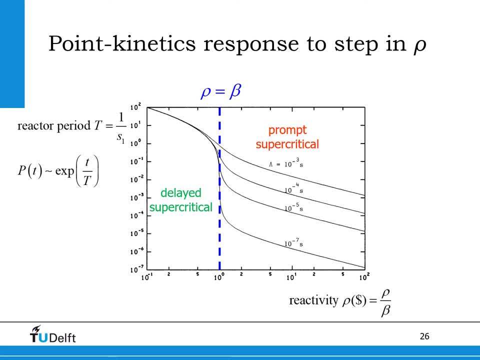 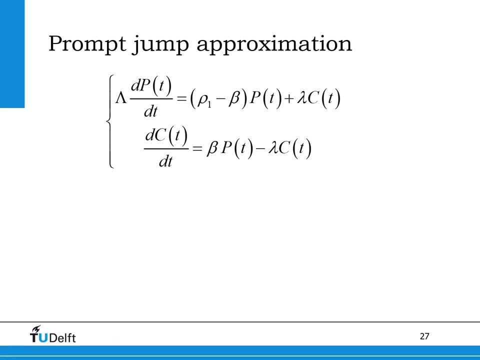 This means the reactor will be very difficult to control and in some cases the automatic feedback effects, like the nuclear Doppler effect, might not be able to compensate for the inserted reactivity. On slide 19 of this presentation, we discussed the solution of the reactor power. 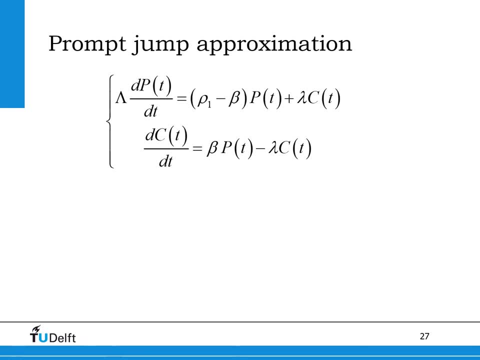 with one lumped family of precursor atoms in play With a positive reactivity step, We saw that the solution was made up of a positive contribution and a small correction to it with a negative sign. The negative part was a function of the neutron generation time. 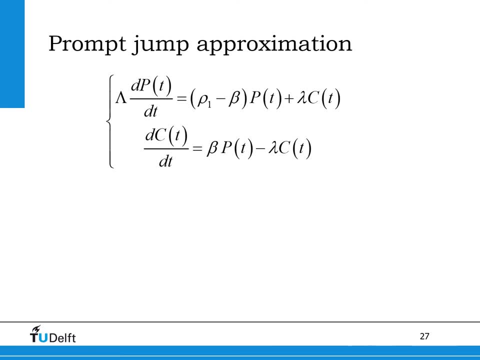 and became zero quickly after the reactivity inserted. Here we will take a look into the solution of the power in case the generation time gets a very small value near to zero On the slide. the point kinetics equations are given for one lumped precursor family. 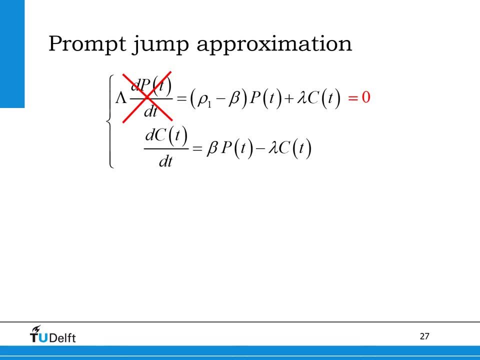 And if the neutron generation time capital lambda goes to zero, the reactor power makes a step, here indicated with the Heaviside function. This means that the derivative of the reactor power just before and just after the reactivity insertion is zero, as shown in the figure. 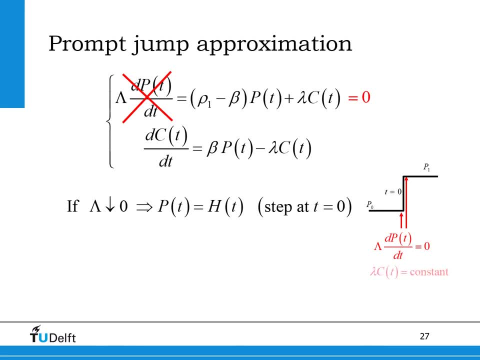 As a result, after a step in reactivity, the power increase is proportional to the ratio of beta minus rho after and before the reactivity step. This is shown in the red formula in the box and is called the Brom-Jump approximation to the solution of the point. kinetics equations. 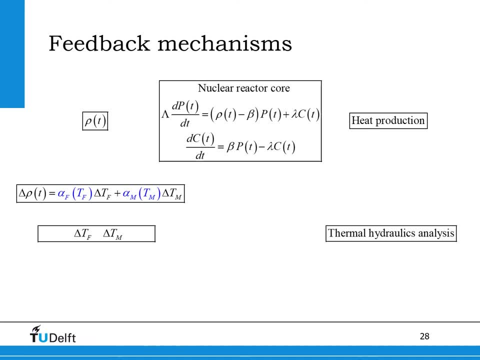 In this lecture we have presented the point kinetics equations and we found an expression for the reactor period characterizing the change in power of the nuclear reactor. In reality, the dynamics of a nuclear reactor will not follow the derived kinetics behavior due to the automatic feedback effects. 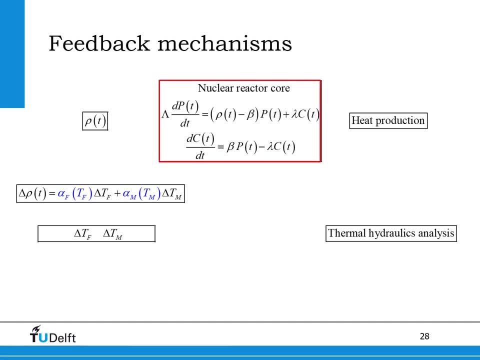 Imagine we have a nuclear reactor core with a fission neutron production rate B as a function of time, with the reactivity as input, Because a fission neutron production rate and the heat production rate in the core are linearly related to each other. 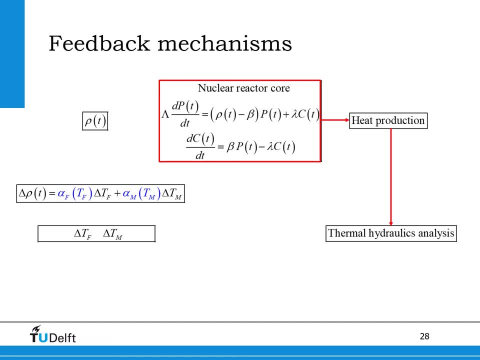 we can easily express the heat produced in the reactor core as a function of P A. change in heat production leads, via a thermo-hydraulics model, to a change in the temperature of the fuel and moderator, Through the nuclear Doppler effect for the fuel temperature. 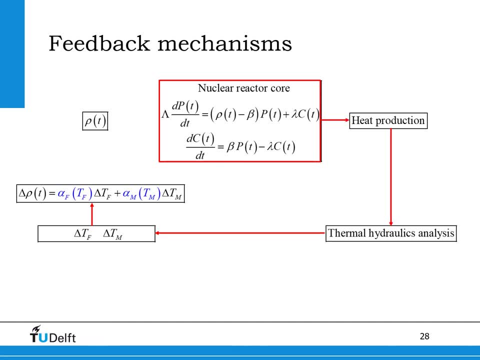 and the dependence of the macroscopic cross-section on the density of the moderator. the reactivity of the reactor core depends on the fuel and moderator temperature as well, And the blue alpha terms in the box are called the reactivity feedback coefficients and can be defined for the fuel temperature. 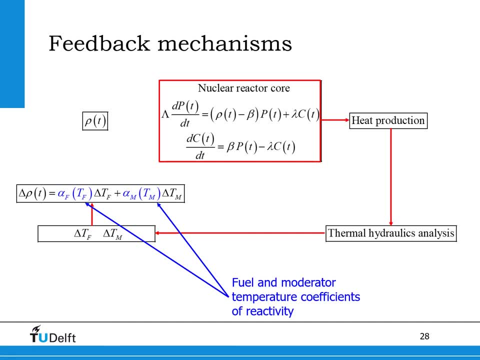 for the moderator temperature, but also for the temperature of structural materials, the coolant and other agents if needed. When the change in temperature changes the reactivity, the power of the nuclear reactor will change as well. Clearly, when the value of the reactivity feedback coefficients 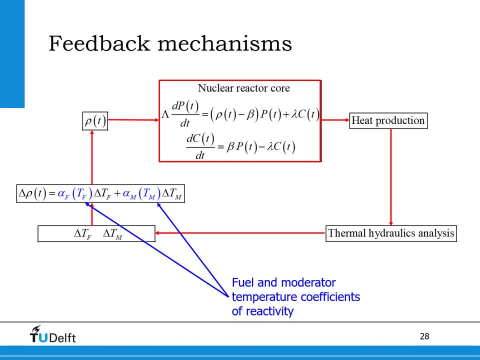 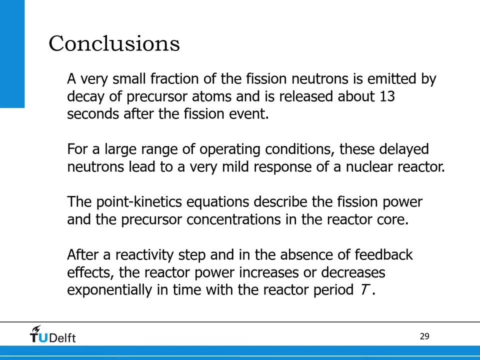 are negative, the reactivity of the reactor will always automatically return to zero and the reactor will reach a new stationary state. We will finalize this lecture with a number of conclusions. First, we've seen that a very small fraction of the fission neutrons 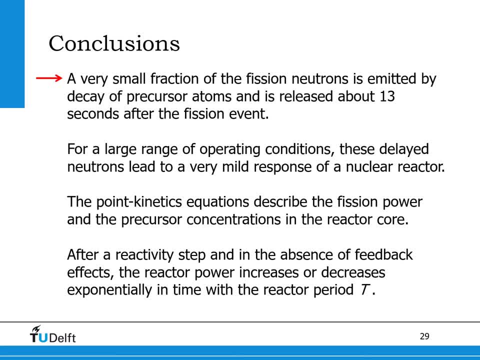 is emitted by decay of precursor atoms, and this fraction is released about 13 seconds after the fission event. For a large range of operating conditions, these delayed neutrons lead actually to a very mild response of a nuclear reactor And the point kinetics equations derived here